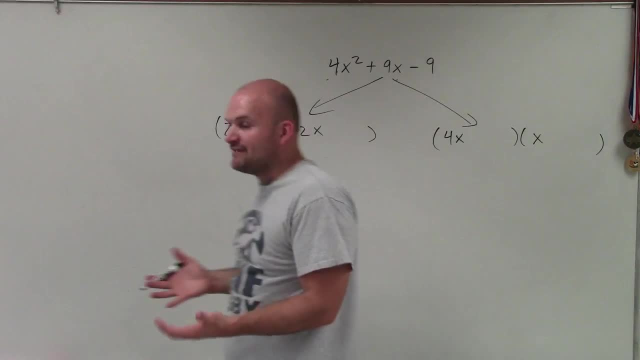 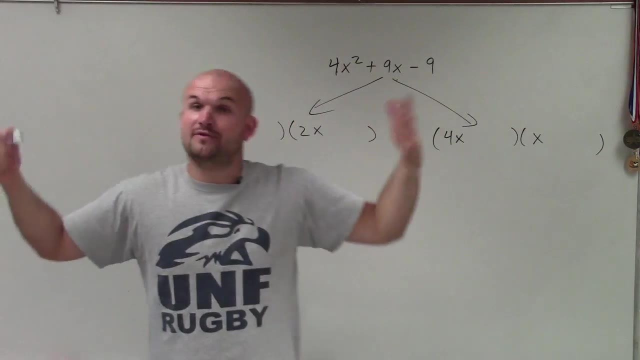 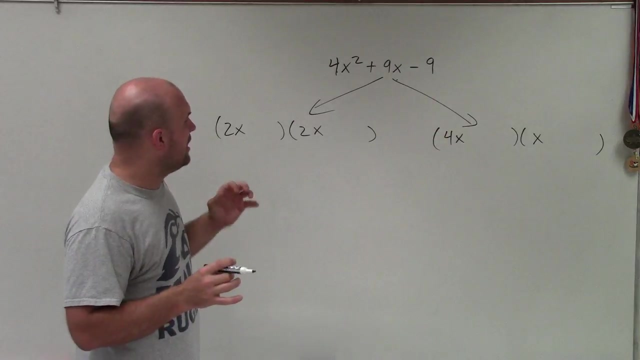 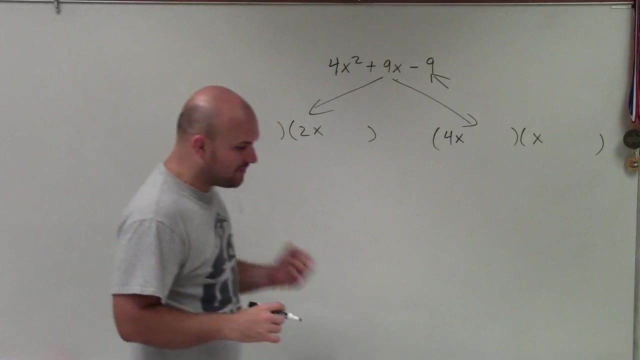 Or I could do 4x times x, right? Those are my two kind of options. And if you have any other number as in front of here, then let's say it was like 12.. Well then you'd have a lot of different options, right? So mentally, all right, I'm thinking: OK, So these two numbers have to multiply to give me 4x. And then, remember, they also have to multiply to give me 9,, these last two numbers. So remember, if they're multiplying to give me 9,, one factor has to be positive, one factor has to be negative, which is even making this even better. 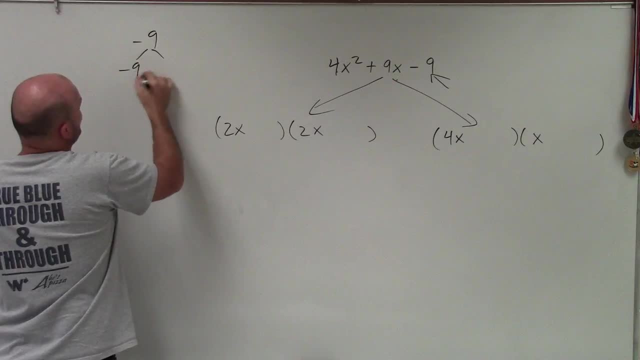 So let's write down the factors of negative 9.. I could do negative 9 times 1.. I could do positive 9 times negative 1. I could do negative 3 times 3.. And it really doesn't matter which one's negative, because they're the same number. 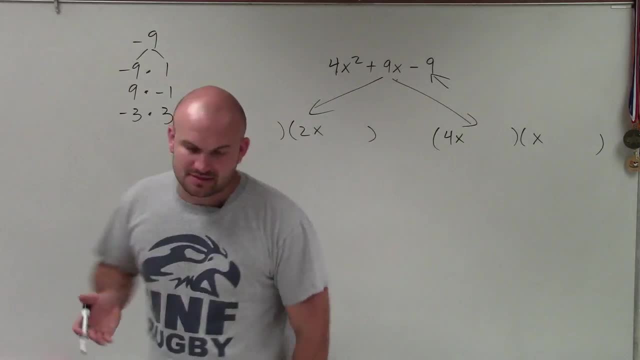 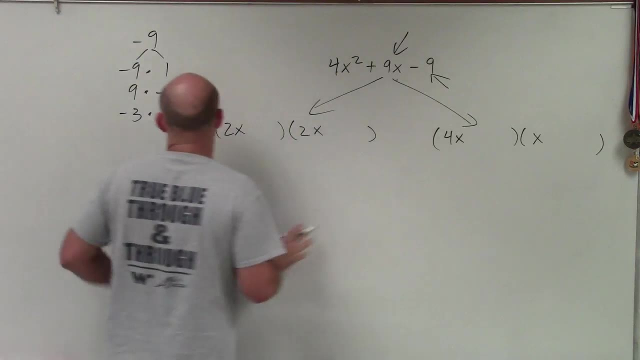 So to think about this, to go through my thinking process, what I'm going to do now is say: all right, well, remember when we got pretty much the last two terms covered in, right, And you could use guess and check if you'd like to. 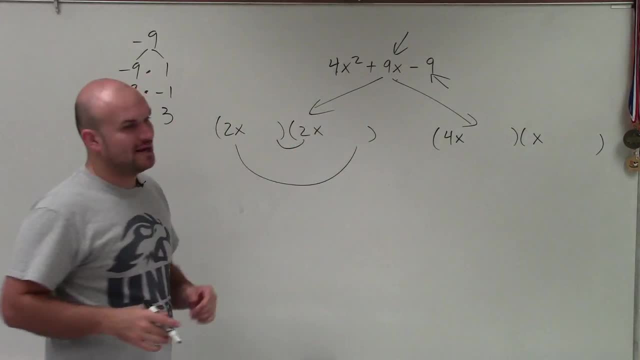 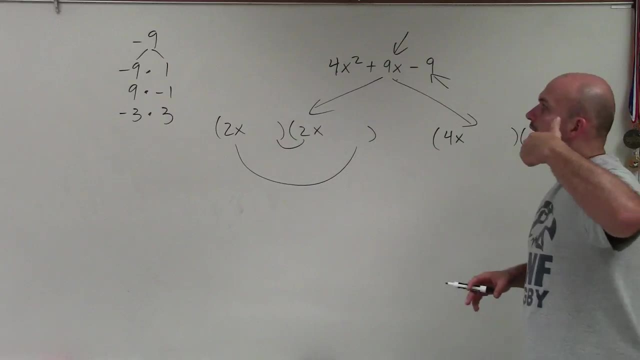 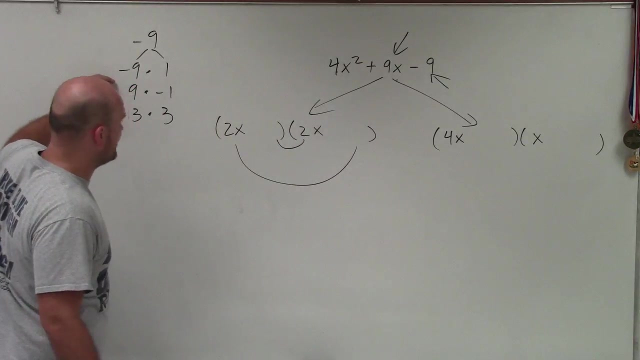 But now what we want to say is: well, what two numbers are going to multiply to give me my out, you know to when I combine, are going to give me a positive 9x. Now, when am I thinking through this? Since they're going to add to give me a positive, I know that the larger of the numbers has to be negative, right? 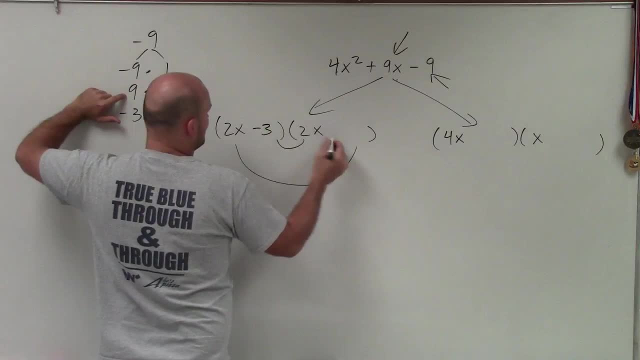 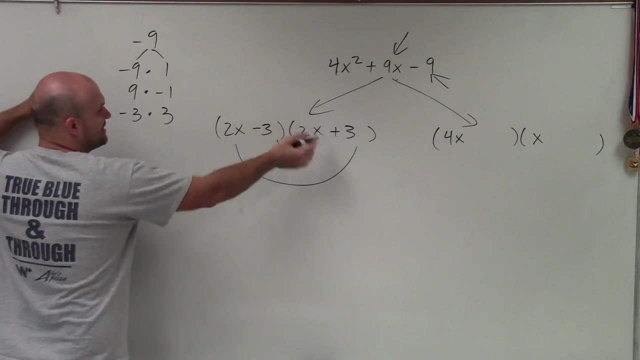 So I see that this is not going to work. negative 3,, positive 3, because this would be like a difference of two squares right? This would just probably: it's 2x times 2x. that gives you negative 9.. 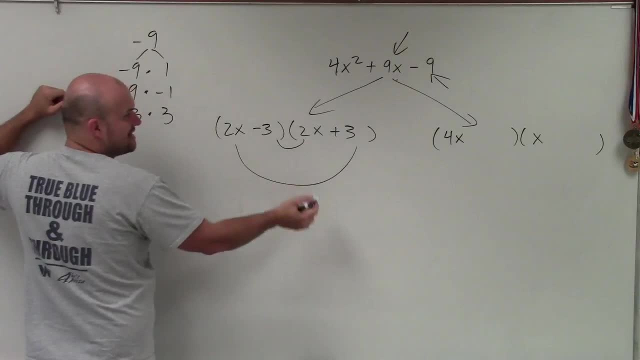 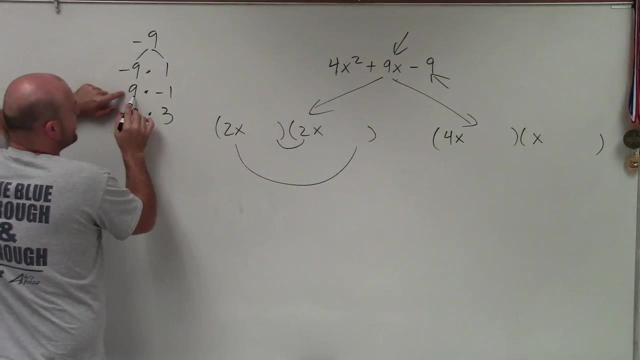 But when you combine these, that's, they're going to give you the exact same answer. So it's going to give you 0x. right, We need to get 9x. So then I look and say, all right, well then, the only other option it could be is positive 9 and negative 1.. 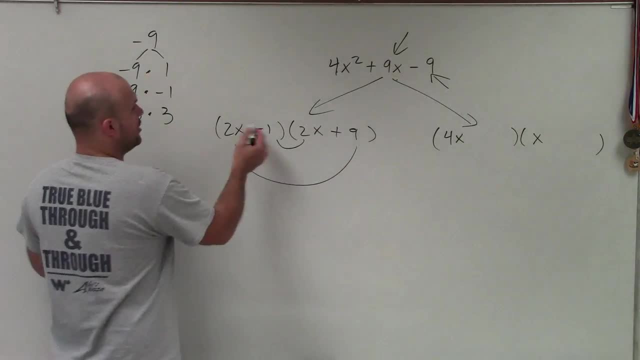 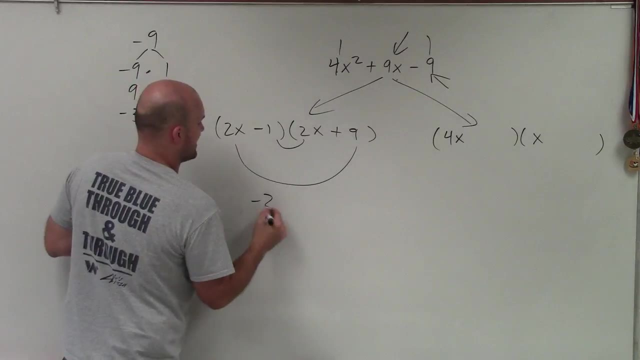 And again, it doesn't matter which way you put them in there. So we know that again, the first and the last give us our two values. But what about the inner? So here I'd have negative 2x, and here I'd have positive 18x.